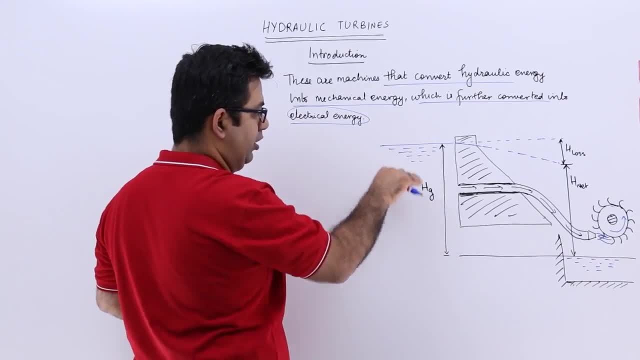 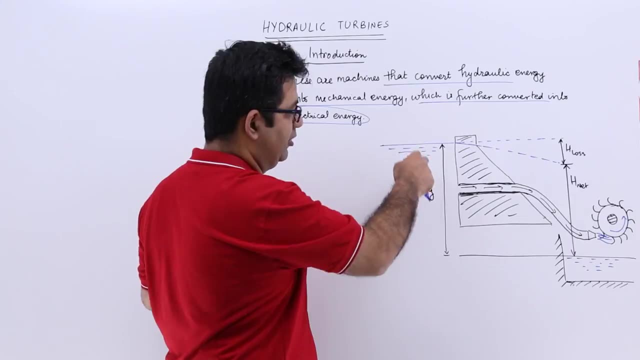 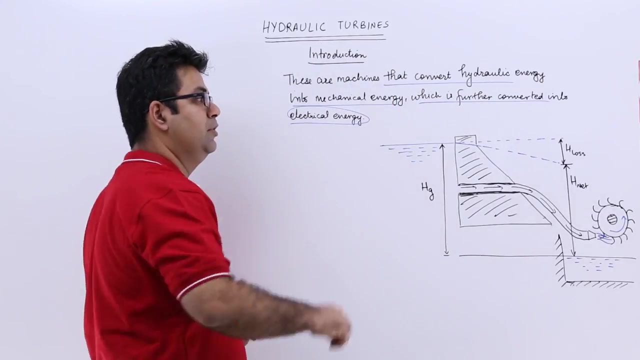 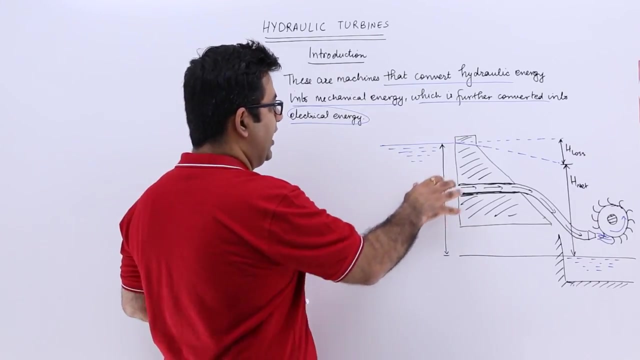 So you have this water which is stored with the help of a dam. It has some height. Because of that height, you have some head of that water. So this is the lowest point in this entire system of turbine. This entire system is called hydroelectric power plant because this hydropower is converted into electrical energy with the help of this turbine. 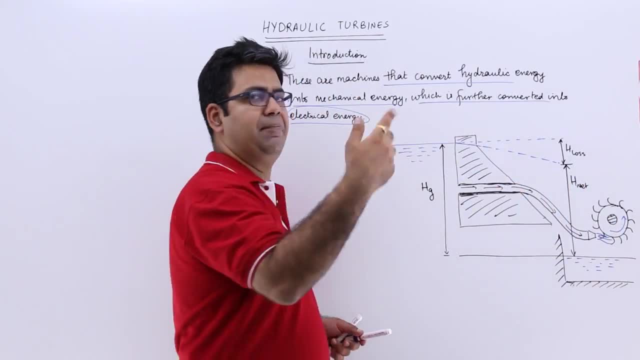 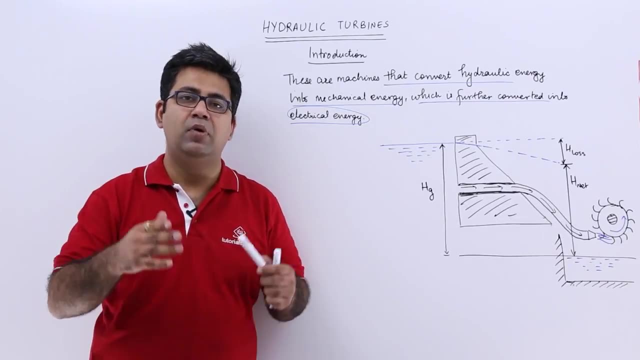 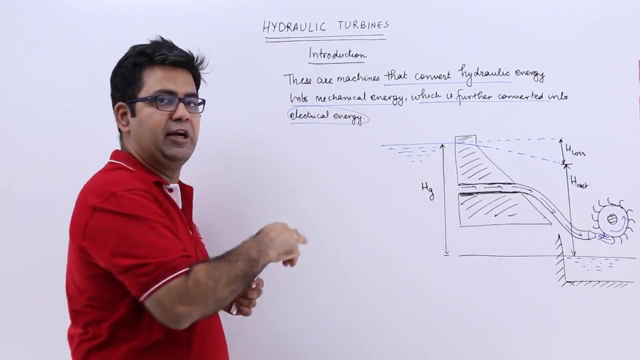 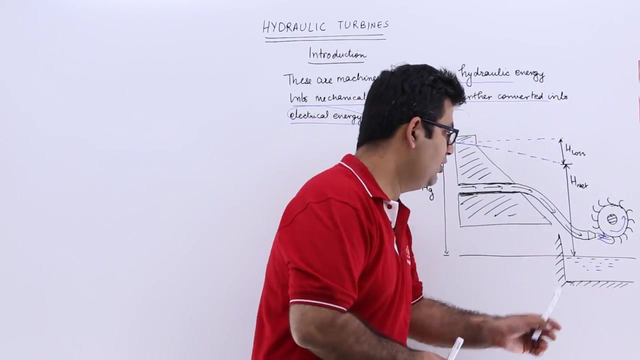 So this turbine is further coupled with the help of a shaft and a coupling, two alternators which produce the electrical energy which is further distributed through grid lines. Now, this is the highest level of the water in the entire system and this is the lowest level. The highest level is called the head race and the lowest level is called the tail race. 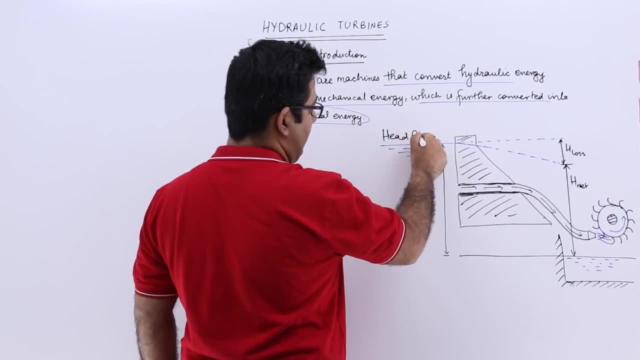 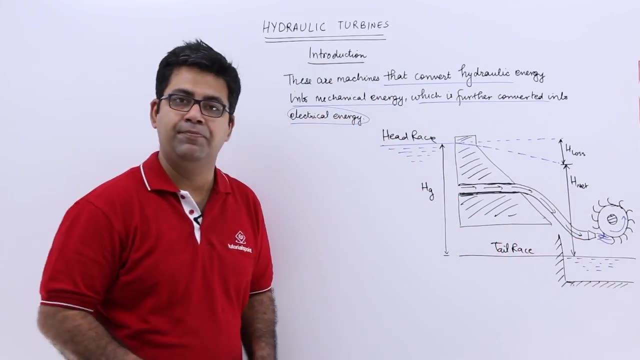 So this is the head race And the lowest level is called the tail race. So what happens is that, let us say the distance between these two races, this liquid column is called the gross head of water, which is available for us to convert into some useful output. 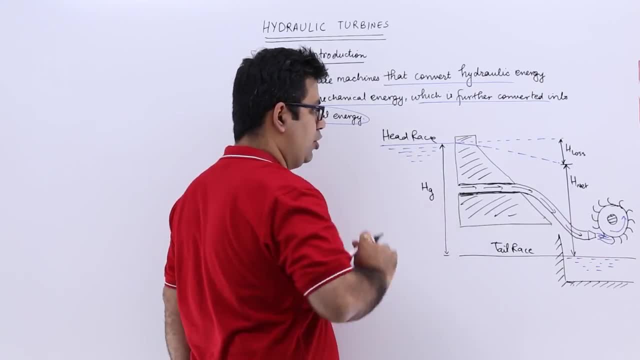 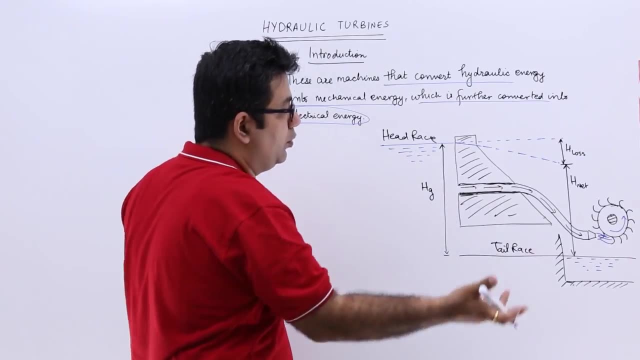 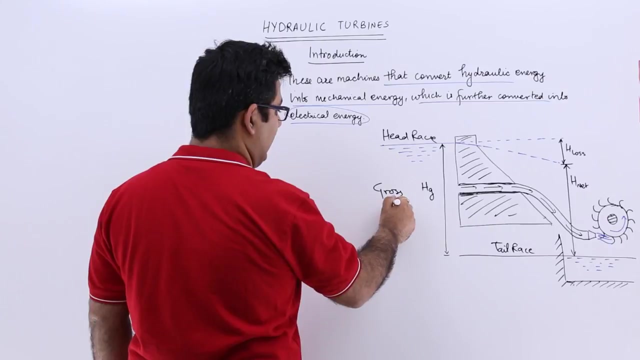 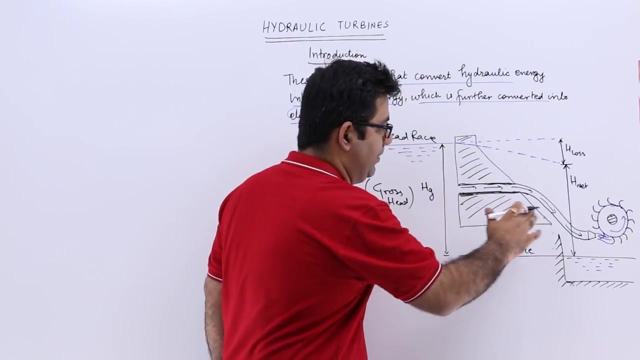 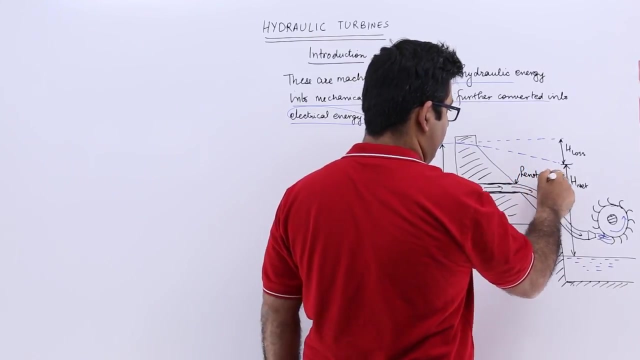 So this is called the gross head of water which is available for us to convert into some useful output. this is called gross head. ok now, as the water flows through this penstock or through this pipeline, so the technical name of this is penstock. ok, so through this penstock, the liquid. 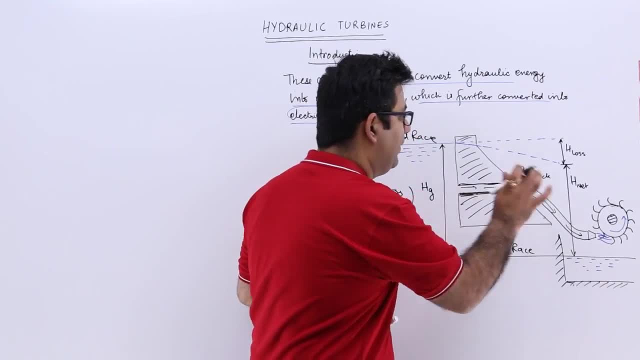 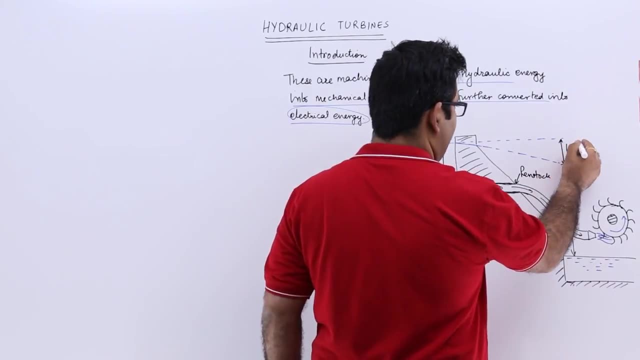 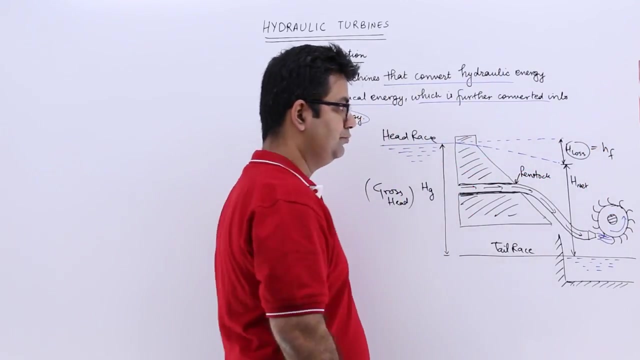 flows and during this flow, that is, flow through a pipeline, there are some frictional losses, there are some leakage losses, ok, so due to that, some head is lost, we will assume it to be friction loss only. ok, and from the gross head, some head is lost due to friction and 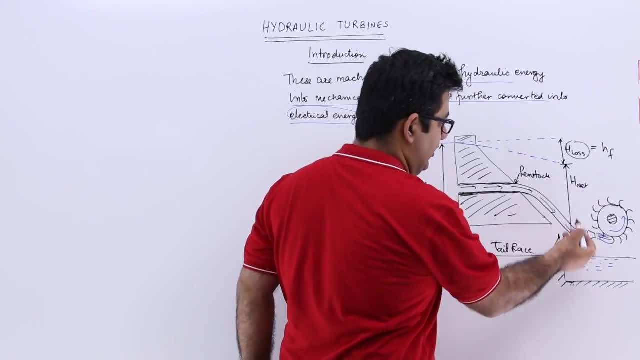 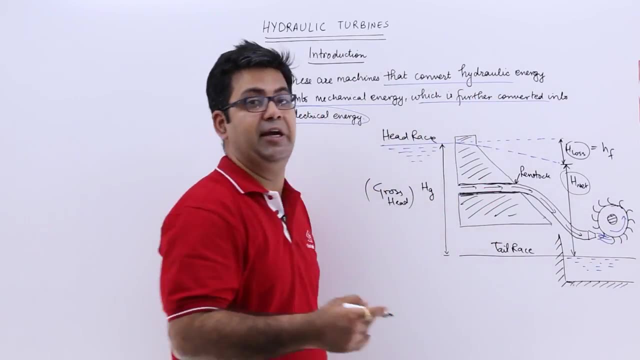 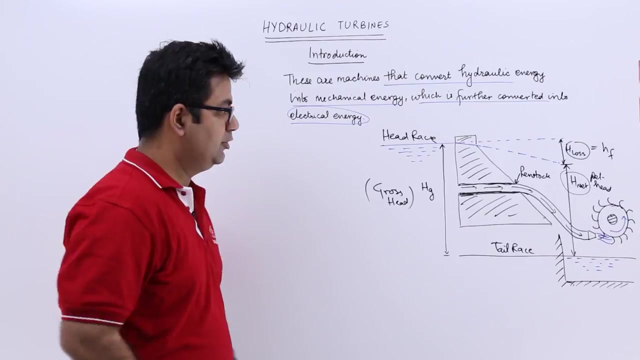 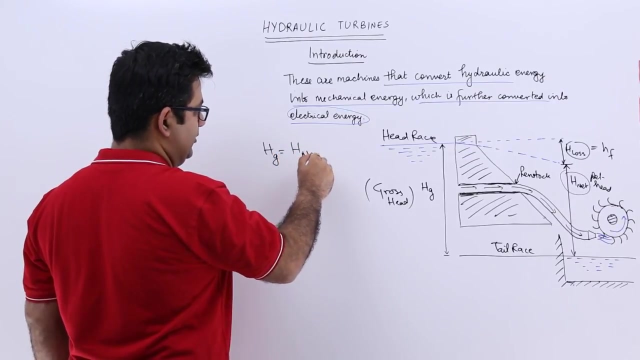 you know, leakage and the head that is left, which is available to us or which is available at the inlet to this turbine, is called the net head. This is gross head. This is gross head. This is the net head. ok, so we can say that gross head is equal to the net head plus the 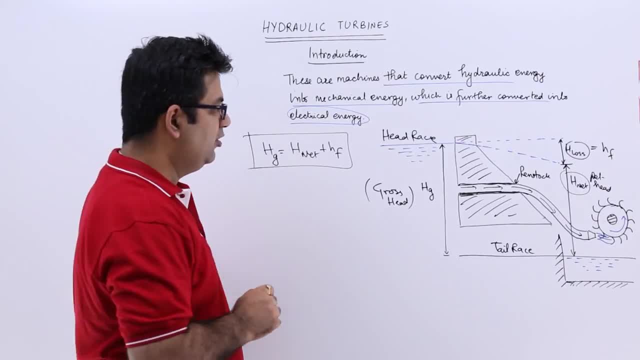 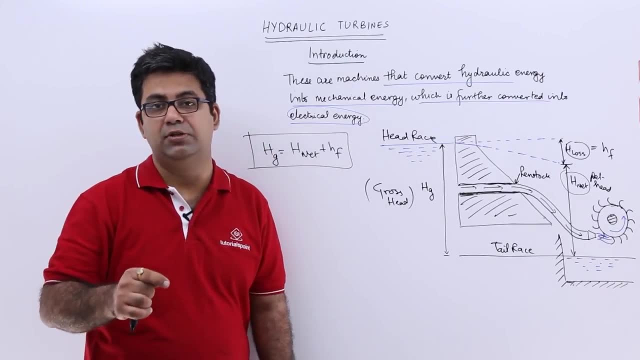 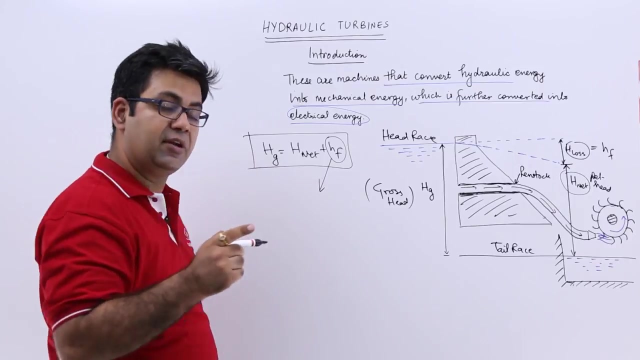 head loss due to friction. alright, so we don't consider the leakage loss a very big loss in such a big system, but the head loss due to friction is of high importance. so what is the value of this head loss due to friction? This head loss due to friction can be found out by using the Darcy-Weisbach equation. so 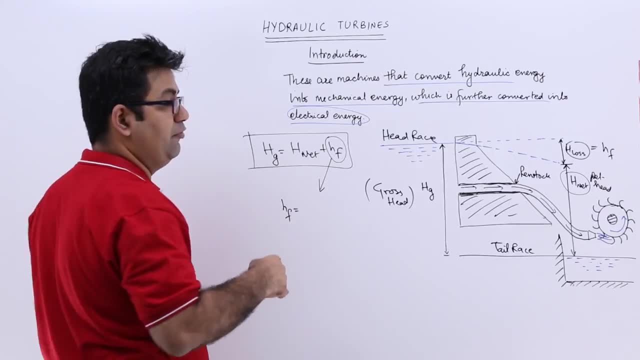 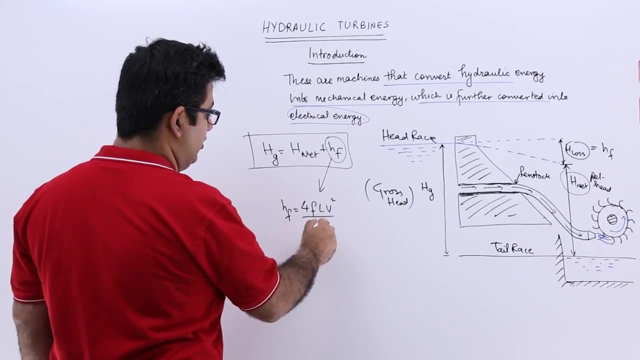 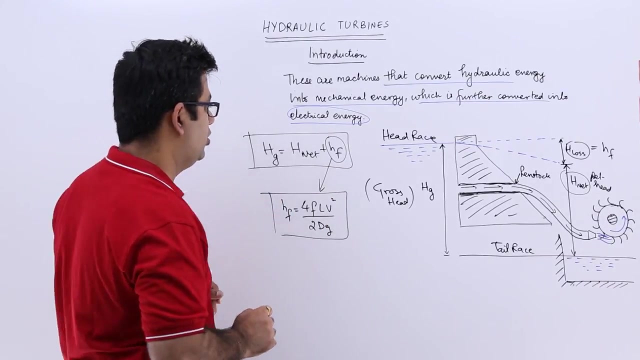 Darcy-Weisbach equation was head loss due to friction in a pipeline which is 4 into f, l, v square upon 2 into d into g. so this is the formula to calculate the friction head loss. ok, so this is a very brief introduction to what the hydraulic turbines are. what do? 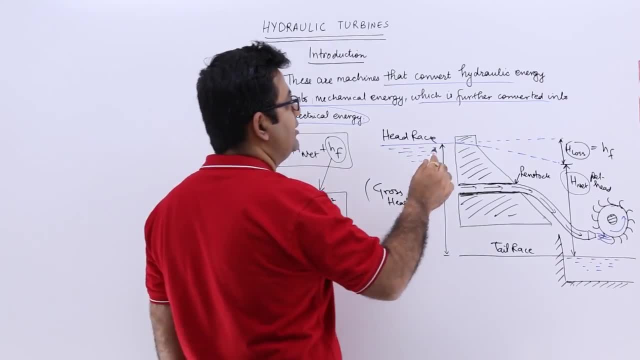 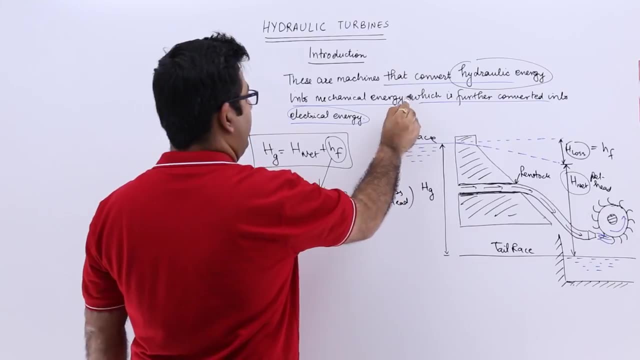 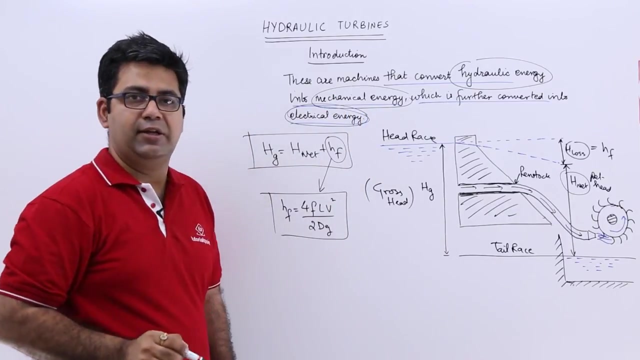 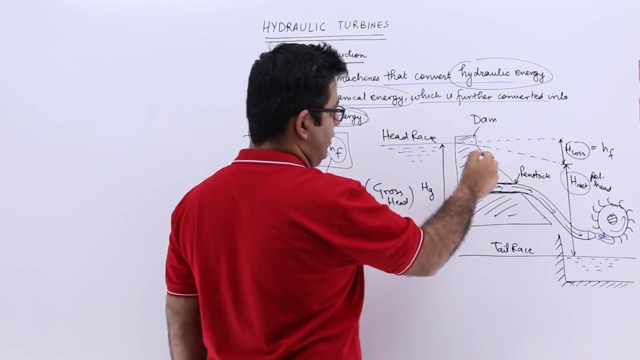 they do. I will just repeat it. I will summarize it: they are energy producing devices. they use the hydraulic energy, convert them into mechanical energy, then mechanical energy converts into the electrical energy with the help of some alternators. so you have a dam. dam becomes the storage of a very big 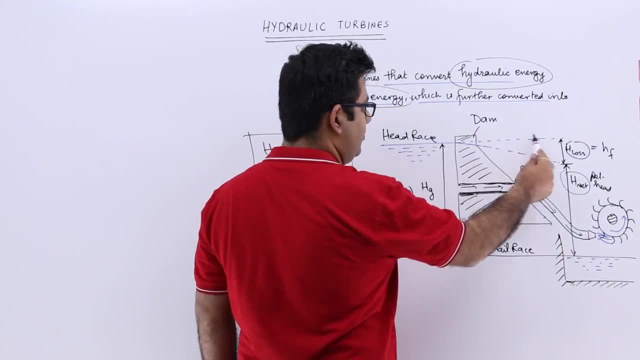 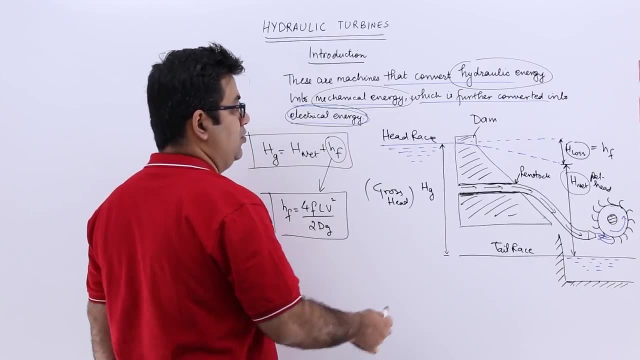 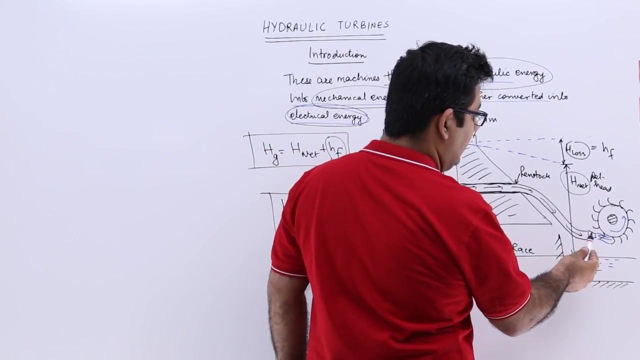 volume of water, The highest point and the lowest point. highest point is called the head race, the lowest point is called the tail race. you have dam, you have penstock or the piping through which the liquid water flows. you have a nozzle. this nozzle directs and controls the rate of flow of water. 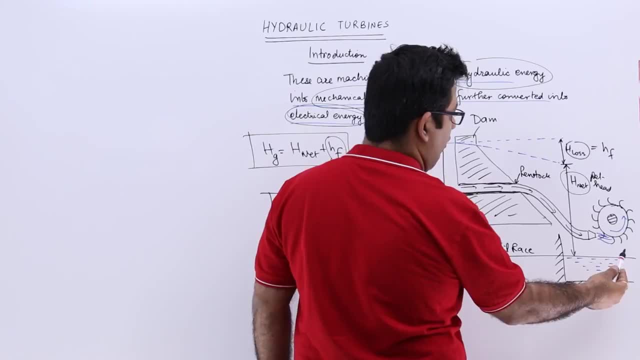 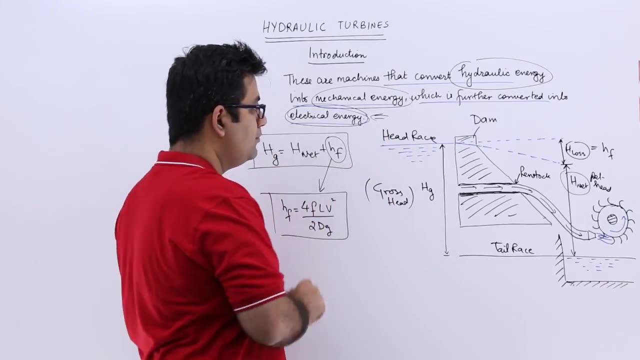 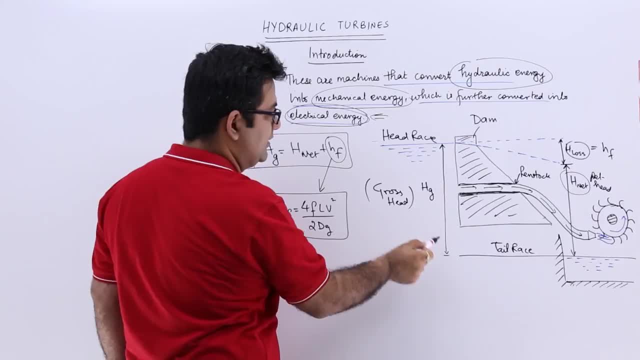 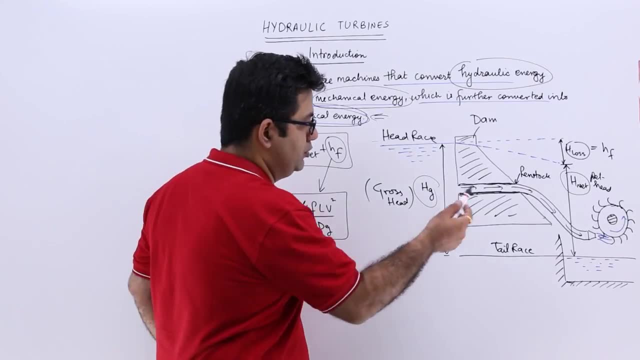 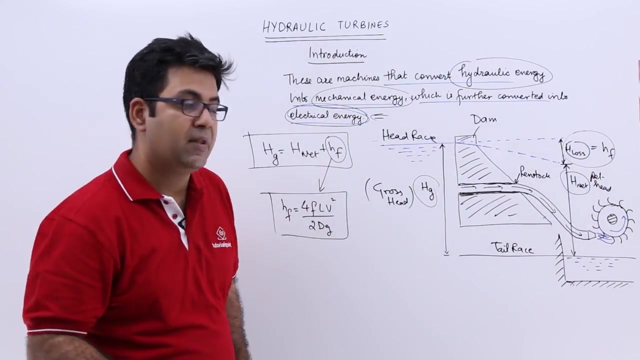 So this is the flow rate of the water. The column of liquid between head race and tail race give you the gross head, that is, the total head that can be utilized to produce the output. but due to the flow in this pipeline, there are losses due to friction and leakage. we mainly consider the friction losses ok.